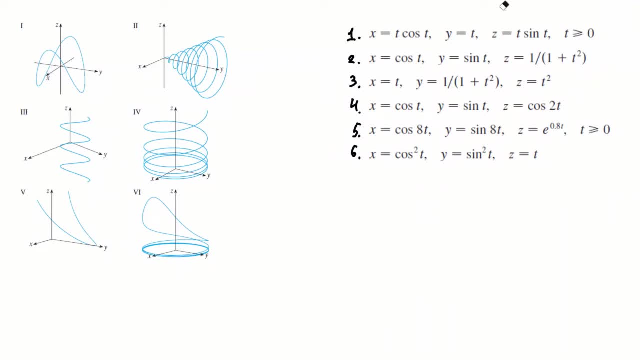 Hello guys, in this video I want to continue covering tricky multivariable calculus problems, and I want to cover this problem which asks us to match the graphs on the left and their corresponding parametric equations on the right. So let's first try to match this first. 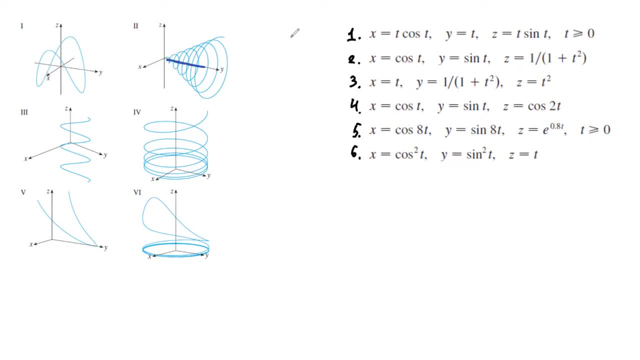 graph. I can see on this graph that my y variable is unbounded. so my variable starts with zero and goes to plus infinity. but for example, if I'm going to take this equation over here, which is equation number six, I can see that my y is going to be bounded between zero and one, since y is 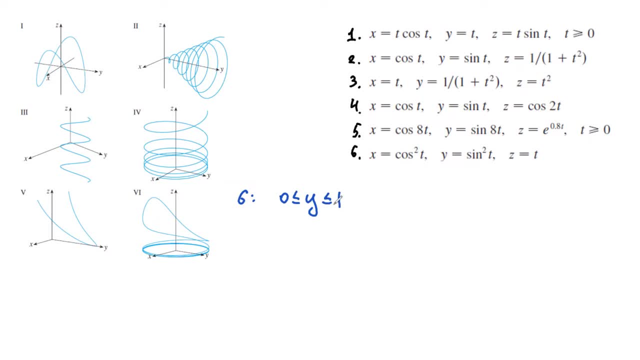 equal to sine squared t. and I know that sine t is between negative one and one. so sine squared t is between zero and one. so that's why equation six for sure doesn't work. for the same reason, equation five doesn't work, because sine of eight is between negative one and one. 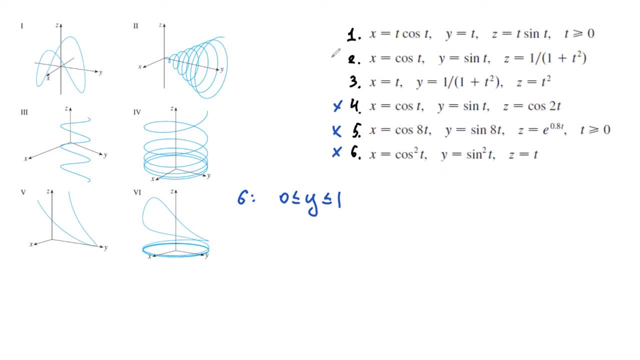 also equation four doesn't work and equation two doesn't work, and again they don't work because in that case my y variable is going to be bounded, but in the graph it's obviously it's not bounded. so the only options are left: equation one and equation three. and how to figure that out? 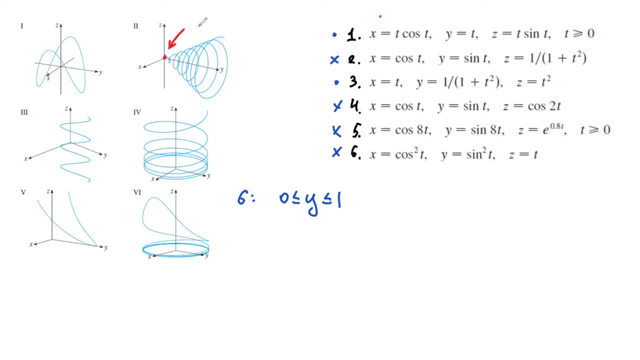 I just need to observe. if I'm going to take the origin point here- zero, zero, zero- then it's going to belong to my graph. so in other words, it means there for this equation, for this equation always must exist some t for which, if I'm going to plug in the 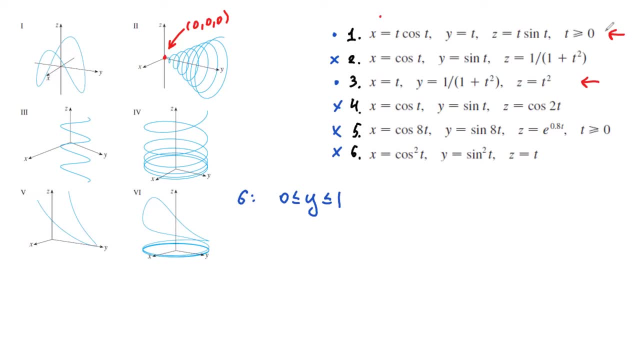 t into my equation, I will get my x component to zero, y component to zero and z component to zero. I can see that for the first equation, t is equal to zero works. so because when t is equal to zero, x, y and z are exactly going to be zero, zero and zero. but what I want to do, I want to make sure that t 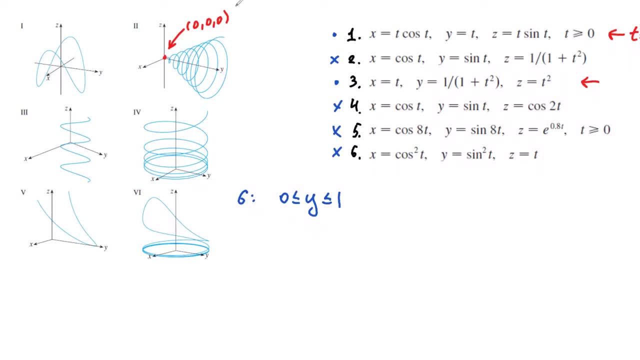 is is that I cannot find such a t that x, y and z at the same time equal to zero for my third equation. so what I'm going to do, I'm going to just try to find such t. so what I want to do, I want to find t such that x is equal. 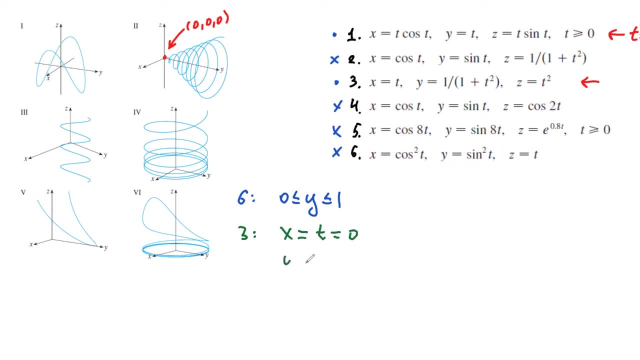 to t is equal to zero, y is equal to one over one plus t squared is equal to zero and z is equal to t. squared is equal to zero. so by solving this equation I can see: obviously t is equal to zero And when I'm going to plug it in into the second equation I will get that 1 over 1 plus 0 is equal to 0.. 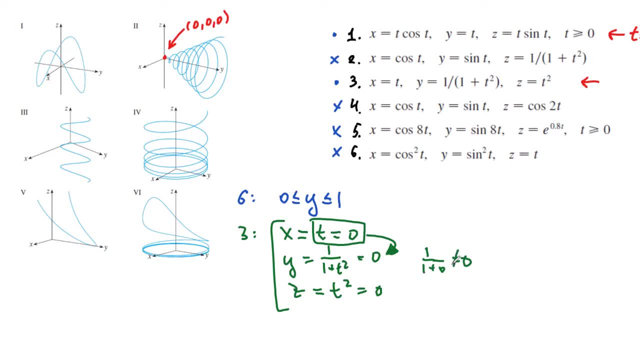 But 1 doesn't equal to 0, so that's why there is no such t, because the only option was t is equal to 0.. Okay so, and we're done with the first graph. We can for sure conclude that graph number 2 is going to correspond to equation 1.. 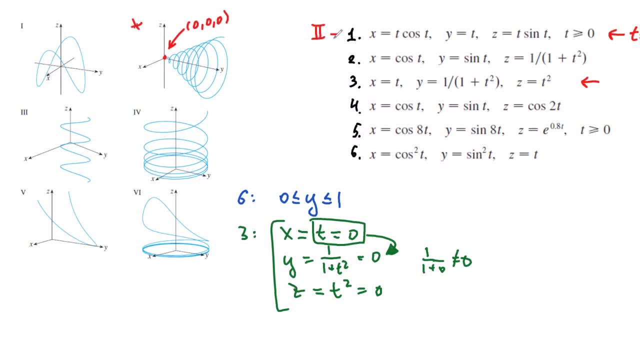 Okay, let's try to figure out other graphs. Let's just take a look and observe to find some properties that we can use. So, for example, if I'm going to take a look at this graph and this graph and this graph, 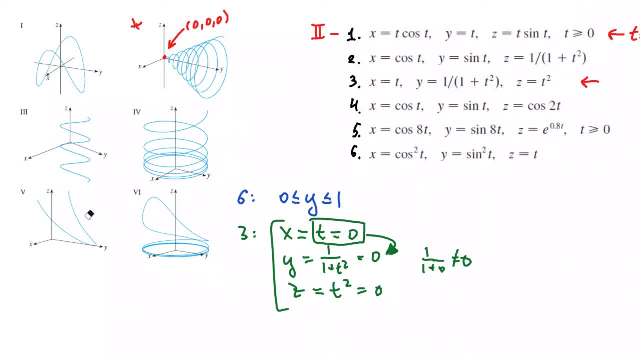 all of those graphs are going to be unbounded, And the only bounded graphs are going to be this graph over here and this graph over here. So, if we're going to take a look at this graph, and we're going to take a look at this graph over here and this graph over here, 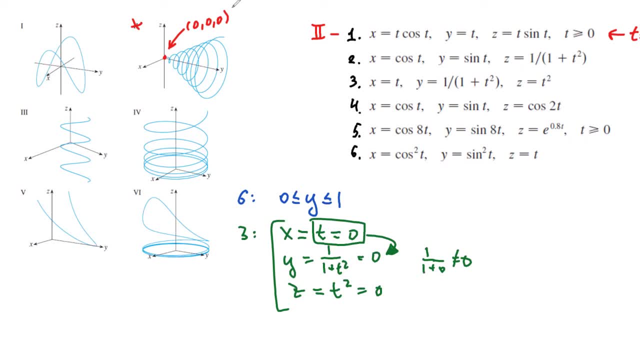 look at these equations over here, then we can observe that if we're going to take equation number four, then for the equation number four x, y and z components are going to be bounded. and the reasons why? because they literally equals to cosine sine and cosine of t, which are between: 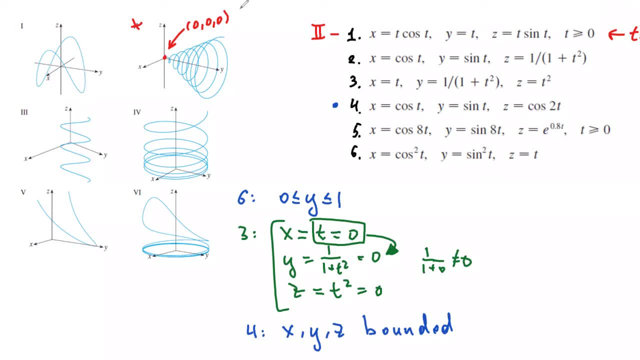 negative, one and one, but i need to decide to which graph this equation is going to correspond to, this one or this one? and the observation that you need to make: that for the equation number six, your z component is strictly bigger or equal to zero, but for your first graph, your z cannot. 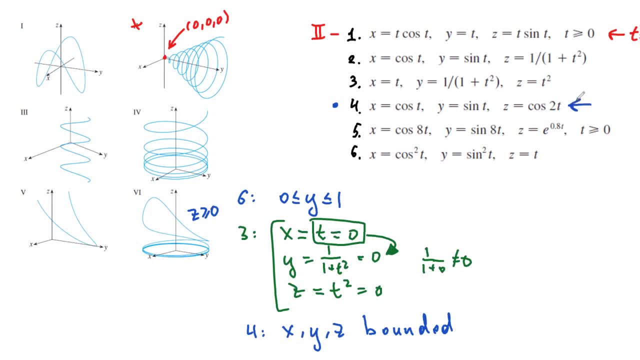 can be negative. and that's why, like your graph, number six doesn't work, because for equation number four, your z component can be positive and negative, since it's equal to cosine of t. so that's why the first graph is going to correspond to equation number four. okay, but then we can observe that, uh then 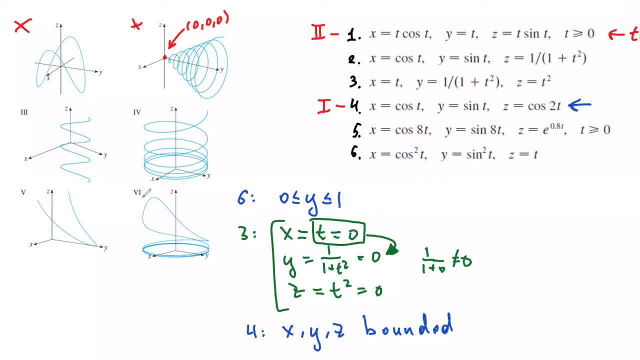 this six graph. number six is going to correspond to equation number uh, q over here. and the reason why is because, uh, all other graphs over here, uh, your z component is here's unbounded. here's z component is unbounded, and here's unbounded means when your parameter t is going to change. 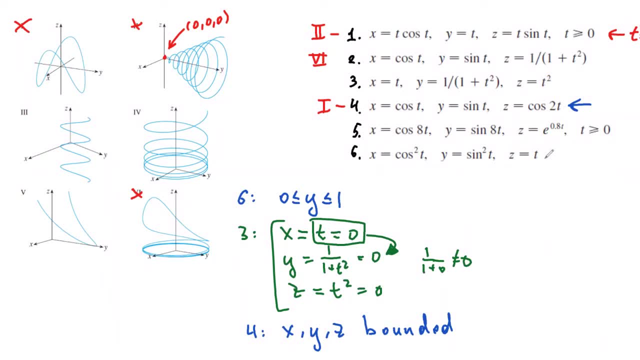 from zero to plus infinity, then definitely t will go to infinity, so z goes to infinity and for all other equation, so the only one a z where your z is uh bounded when t increases, is going to be uh, this equation over here, because when t is getting bigger, bigger and bigger and 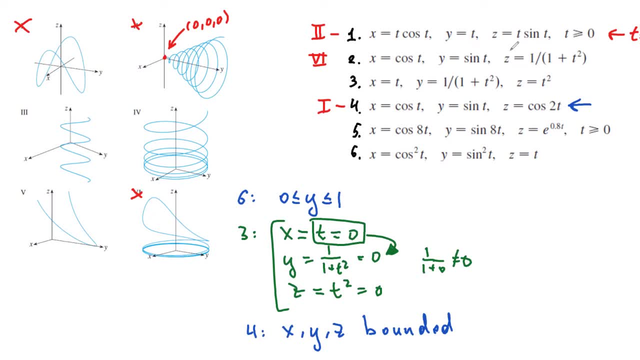 d belongs to uh denominator, then your, you, you. this is going to get smaller, smaller, smaller. and the biggest value of z, by the way, it's when uh t is equal to zero, so z is equal to one. okay, so that's why, uh, we already eliminated uh three graphs. for the next step, let's take a look at this equation over here. 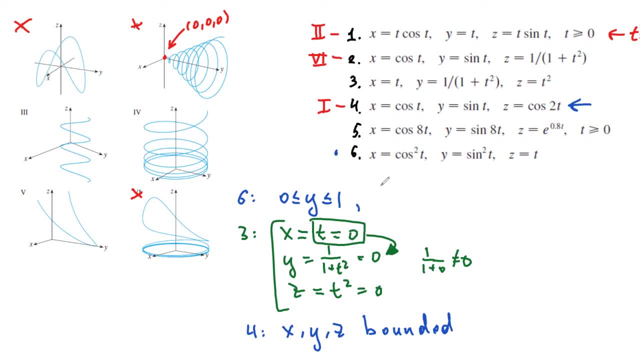 i can see, for the equation number six, my x is strictly bigger than zero and my y is strictly bigger, strictly bigger or equal than zero, because they equal to cosine square and sine square, t correspondingly. and for this graph over here, your x and y- uh, allow it to be negative. 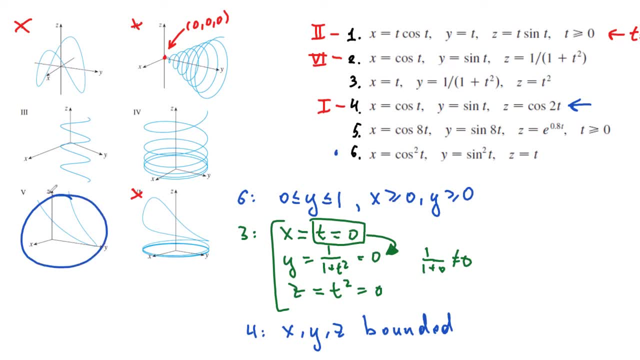 uh for this graph over here. if you will take this branch, this branch is going to belong to uh. they have uh space when x is negative, so this graph also doesn't work. so the only graph for which your x and y uh are going to be in the negative is going to be graph. 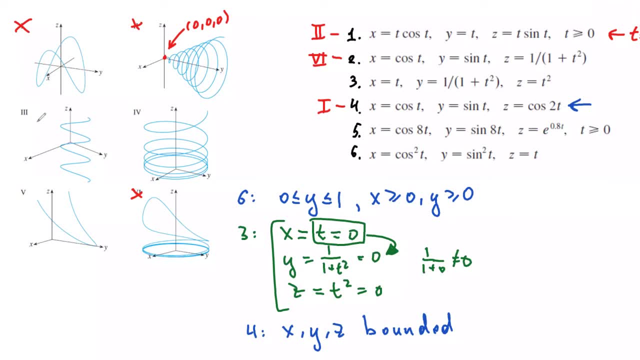 number three over here. so that's why i know that graph number three is going to be equal to the equation six. and finally, we left with two graphs and i need to figure out which of this graph works. and, uh, we can find the difference. for example, uh, when i'm going to take the graph over here. 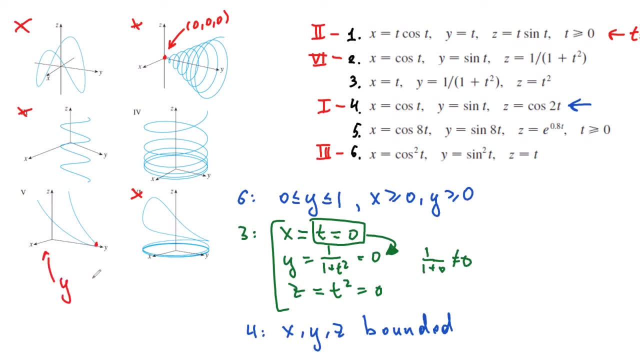 that for this graph over here, my y is strictly bigger, equal than zero. if you're going to take a careful look, when one of the branches getting bigger, big and bigger, it still is going to stay on the positive side of y. and, and here you can see, we need to choose.